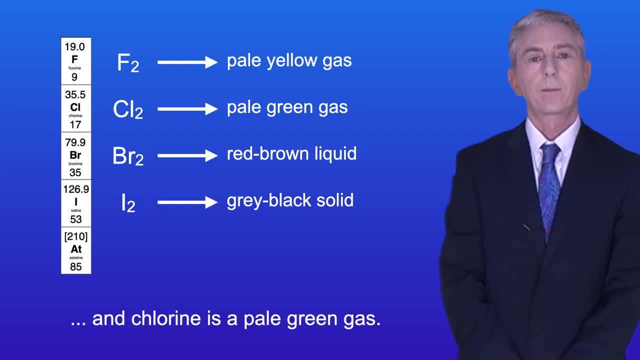 yellow gas and chlorine is a pale green gas, Bromine is a red-brown liquid and iodine is a grey-black solid. Astatine is highly radioactive and has never been observed. We won't be looking at astatine in this topic. 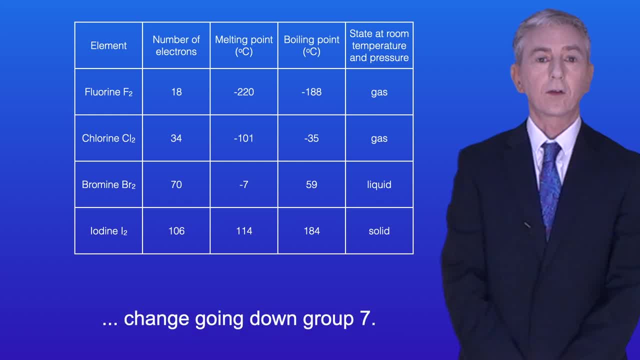 I'm showing you here how the melting and boiling points of the halogens change, going down Group 7.. As you can see, both the melting point and the boiling point increase as we move down Group 7.. Now, in order to explain this, we need to look at the intermolecular 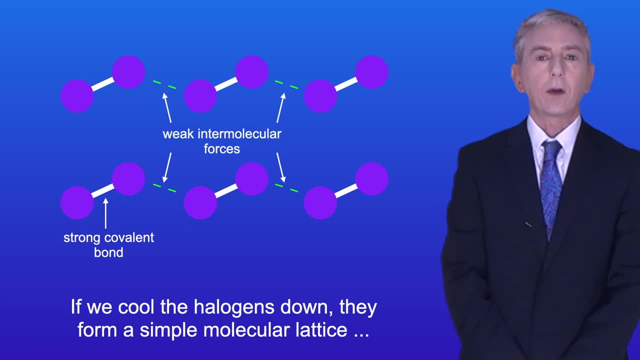 forces involved. If we cool the halogens down, they form a simple molecular lattice, which I'm showing you here. The covalent bond between the two halogen atoms is strong. However, between the halogen molecules, the covalent bond between the two halogen atoms is not. 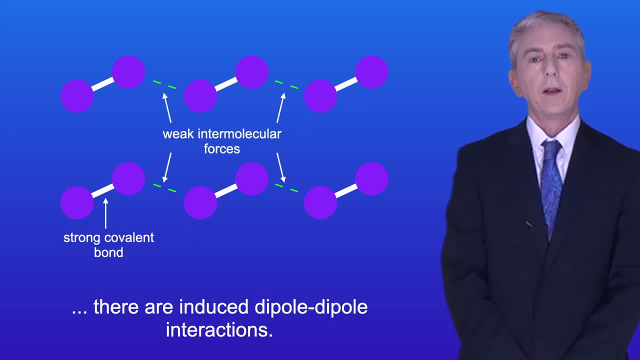 strong. These are the intermolecular forces involved in the melting processes. These are the Mateo molecules that are induced dipole-dipole interactions. These are also called London forces. If you're following the AQA spec, you can call these Van der Waals forces. These intermolecular 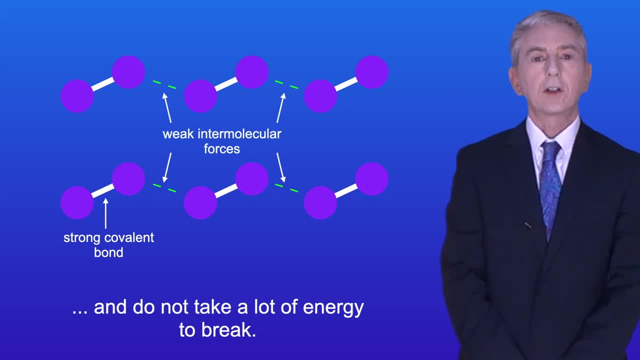 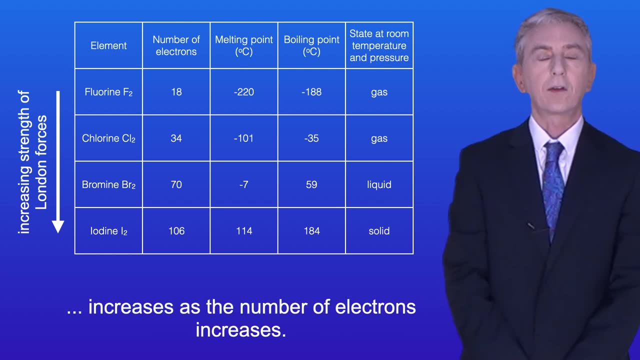 forces are relatively weak and do not take a lot of energy to break. Now you need to remember that the strength of London forces increases as the number of electrons increases. Iodine molecules have 106 electrons, whereas fluorine molecules only have 18 electrons. 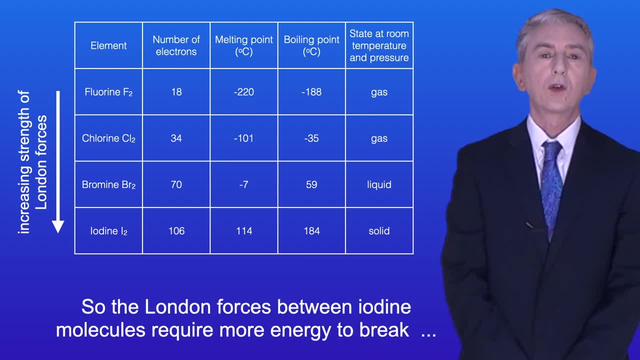 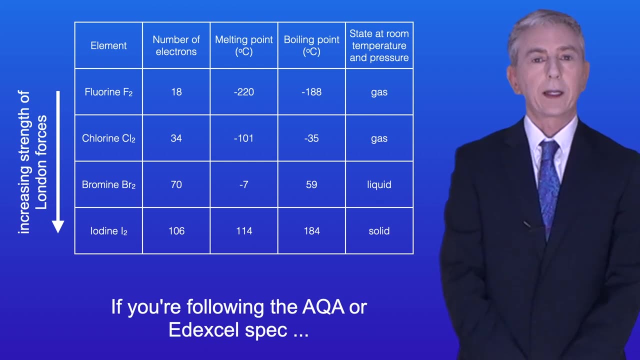 Next slide… electrons, So the London forces between iodine molecules require more energy to break than those between fluorine molecules, and this explains why both the melting and boiling points increase down group 7.. OK now, if you're following the AQA or Edexcel spec, you need to be able to describe the 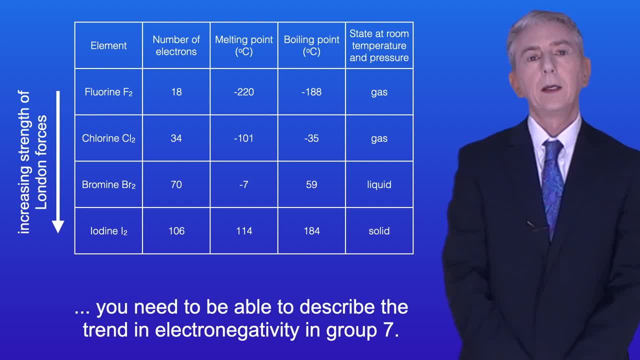 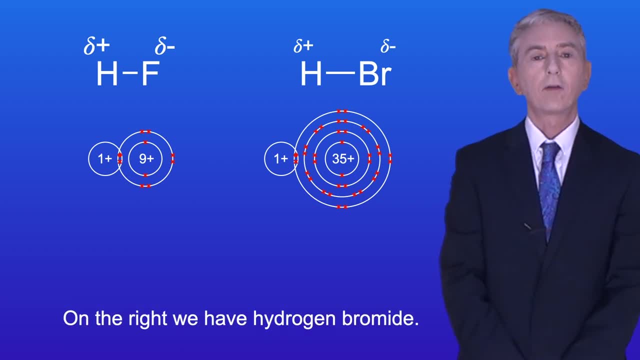 trend in electronegativity in group 7.. I'm showing you here two compounds containing a halogen- On the left we have hydrogen fluoride and on the right we have hydrogen bromide. and I'm showing you the electron shells in these compounds. Now a key idea. 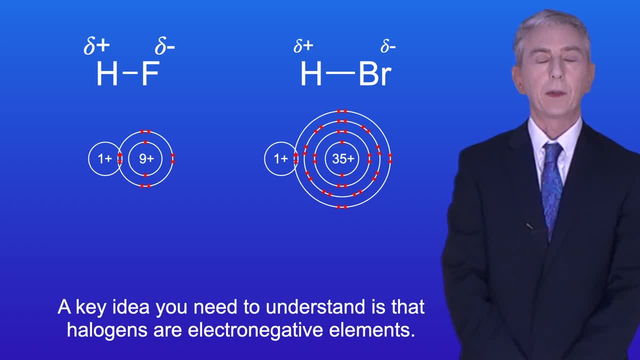 you need to understand is that halogens are electronegative elements and we looked at electronegativity in the topic on bonding. Electronegativity is the ability of an atom to attract the bonding electrons in a covalent bond. Looking at hydrogen fluoride, the fluorine,